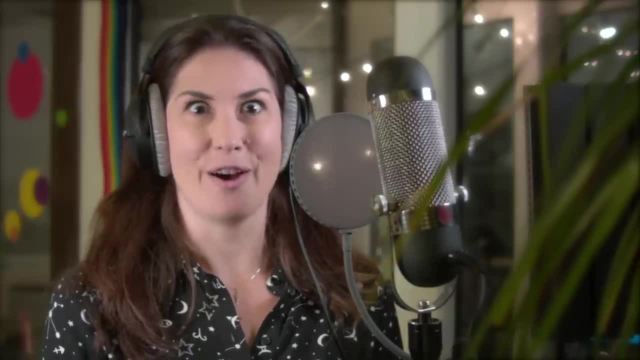 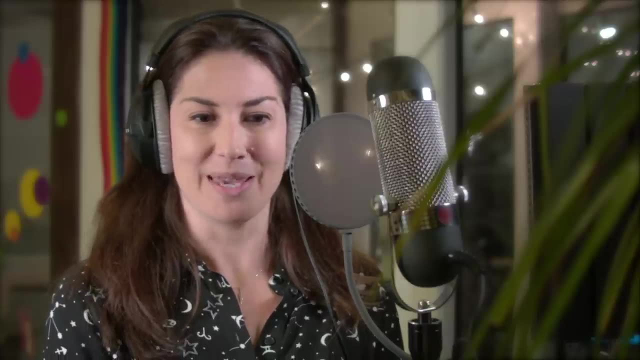 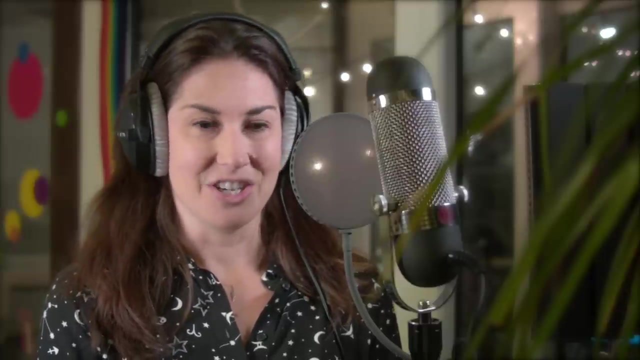 can follow by stretching yourself up as far as you can reach, like you are the flower growing. Then you'll be curling back up again into your little seed shape. Before we start, while you're in your seed shape, take a moment to get comfy so you can. 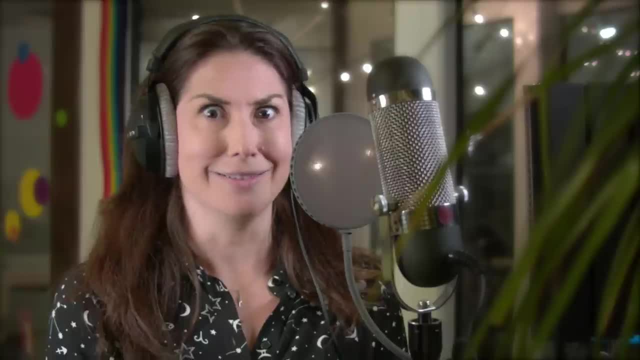 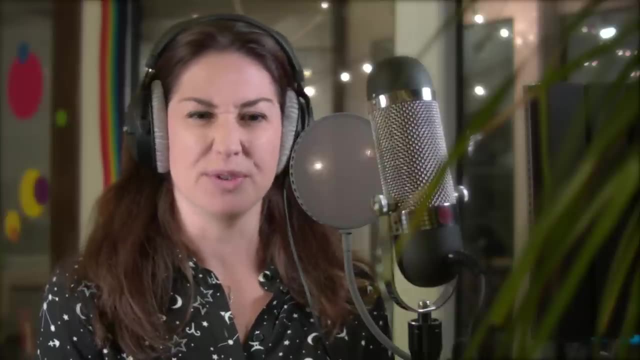 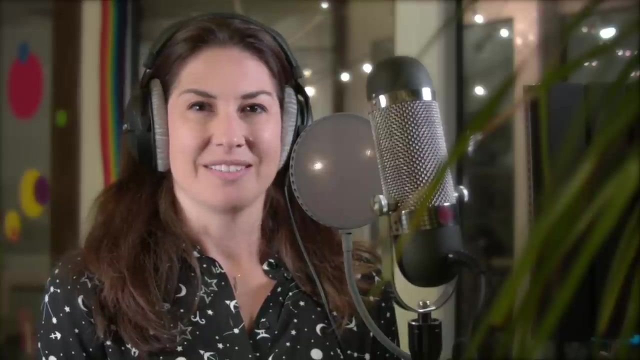 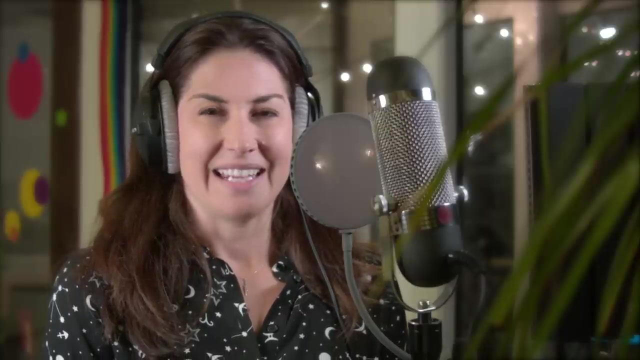 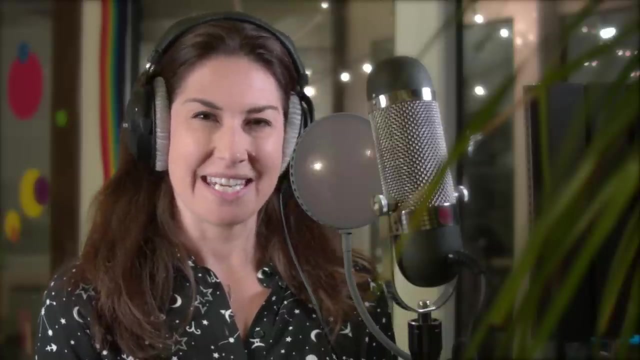 be a very still and quiet little seed. Once you're comfy and you've done any last minute wriggles or fidgets, take a deep breath in, then out And again in And out. Carry on with your breathing, seeing if you can feel the breath coming in and going. 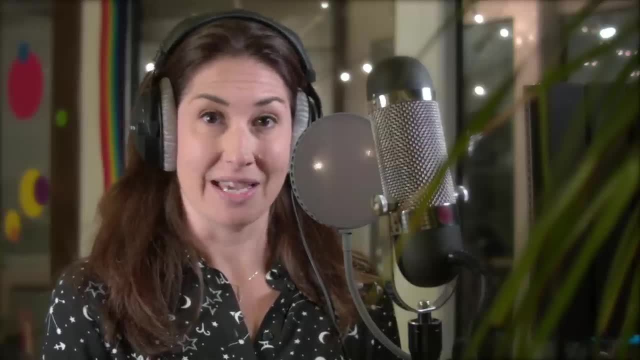 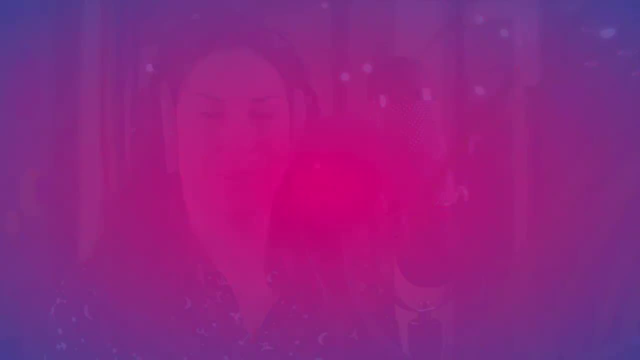 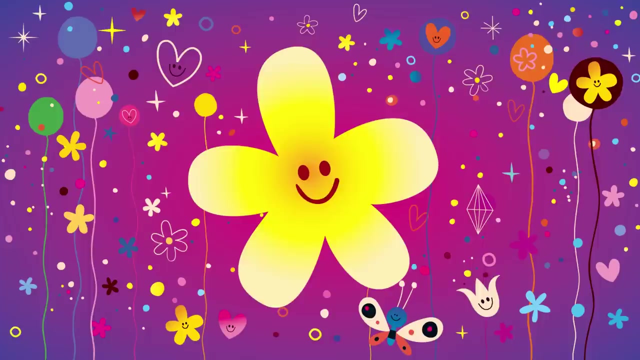 out Next time as you breathe out. if you haven't already let your eyes softly close, Now see if you can follow along. Imagine you are a very little seed, all curled up waiting to grow. You're planted in the 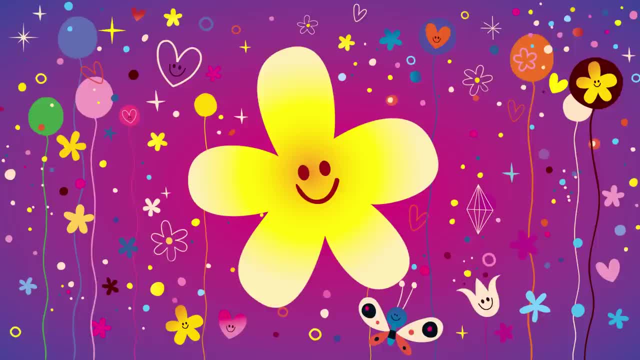 soft brown earth and feel very snug and warm in here. It's especially cosy right now, as it's raining and you can hear the pitter patter of the rain on the earth above you. Slowly the rain clears up and you're ready to go. Imagine you are a very little seed. 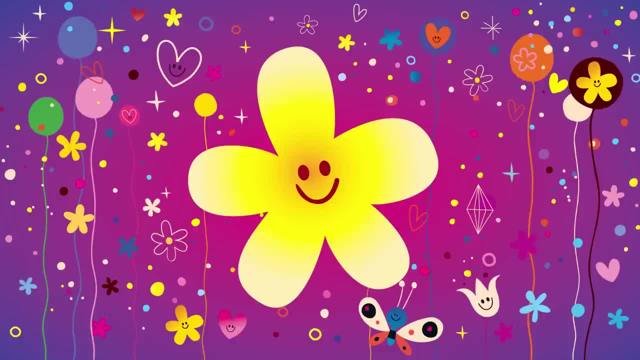 all curled up waiting to grow. You're planted in the soft brown earth and feel very snug in here. It's especially cosy right now as it's raining and you're waiting to grow And you feel the warmth of the sun shining down on the earth above you. It feels so toasty. 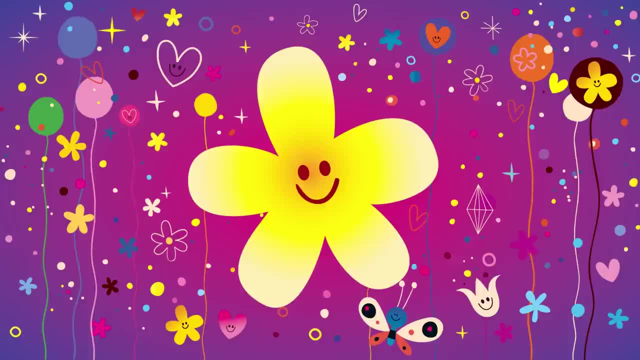 You can feel the sunlight inviting you to stretch up and enjoy its warmth. ava toone, do l righteous work. so you begin to grow, So very, very slowly, inch by inch, bit by bit. Now you are a little green shoot, You've popped up through the earth and the sun is making you feel stronger by the second. You keep on growing, Grow, grow, grow up even further, so your leaves begin to open all the way out, all the way down your long stem. 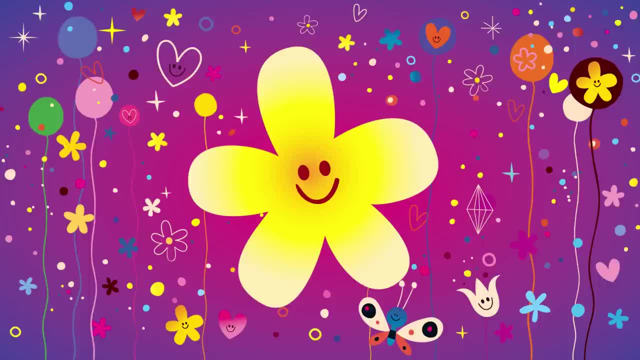 The sun is still beaming down on you, filling you with a shiny, smiley sunshine. feeling You open out into a flower with big yellow petals, A beautiful yellow flower. Even more, you stretch up as if you're trying to reach the sun, Feeling its power, warm your petals. 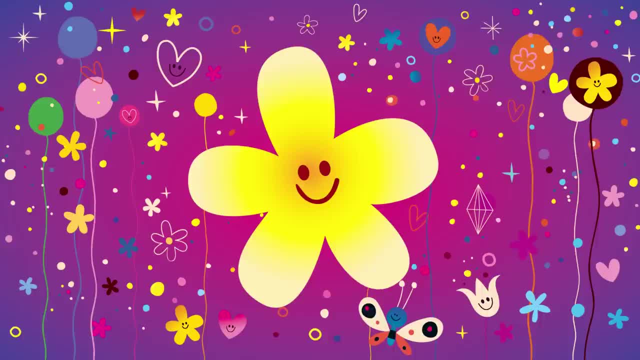 Your leaves, your stem. Slowly. the sun begins to lower in the sky, The day is nearly over, The freshness of the evening draws in and you begin to roll and curl up slowly, slowly, so very slowly, back into your little ball shape. 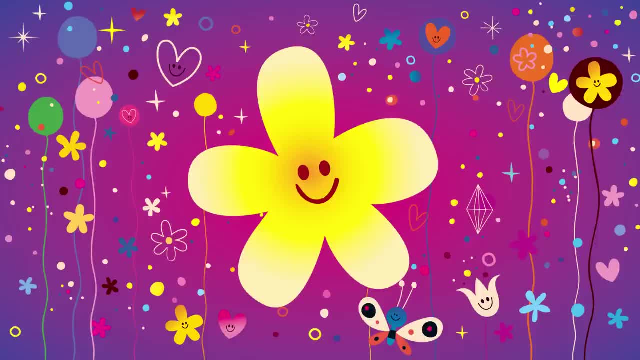 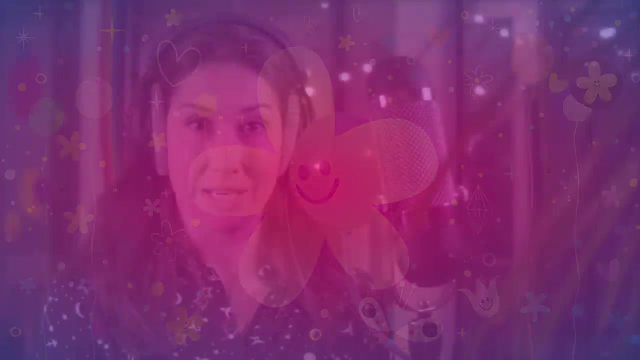 Just like a tiny, tiny ball. Just like a tiny, tiny ball. What a magic feeling it is to grow in the sun, just like a flower. Slowly, now we start to come back, deepening your breath, starting to move your fingers and toes, slowly, gently opening your eyes. 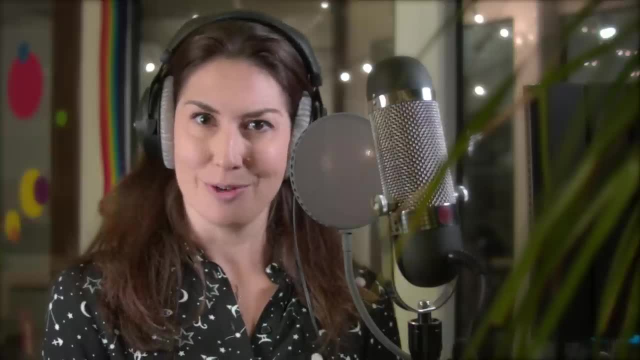 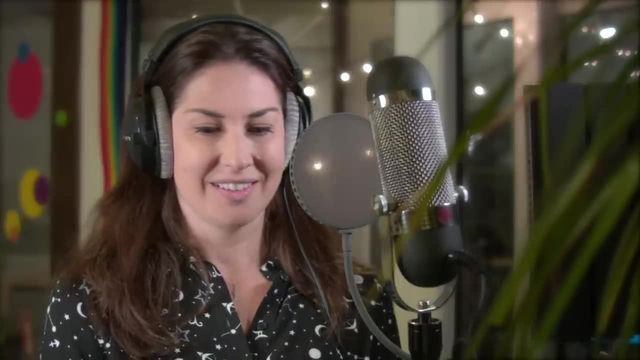 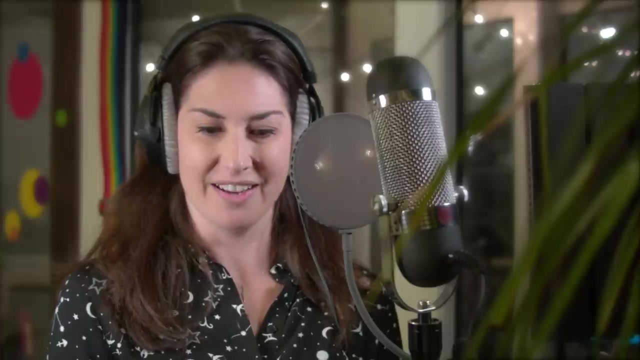 Before you move, just take a moment to notice. This is how you feel now, Different to how you felt before your peace out. Well done you for imagining being a flower and enjoying all that warmth and strength from the sun to make you grow.